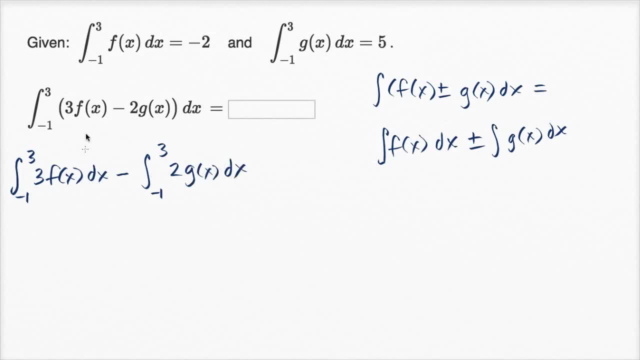 of two, g of x, dx. Notice, all is I did is I split it up. Taking the integral of the difference of these functions is the same thing as taking the difference of the integrals of those functions. Now the next thing we can do is we can. 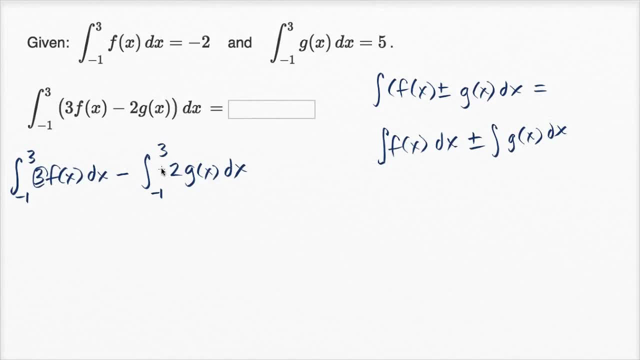 If we take the scalars, we're multiplying the functions on the inside by these numbers three and two and we can take those outside of the integral And that comes straight out of the property that, if I'm taking the integral of some constant. 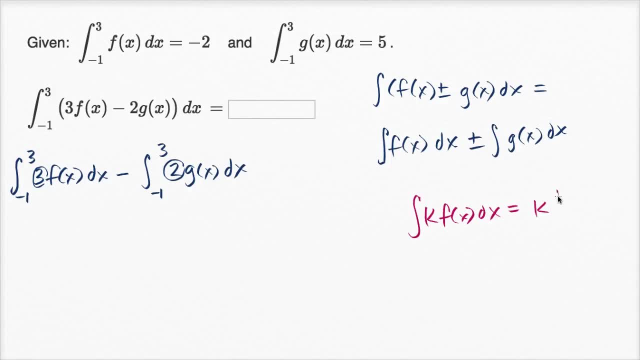 times f of x dx, that is equal to the constant times, the integral of f of x dx, And so I can rewrite this as so. let's see, I can rewrite this first integral as three times the definite integral, from negative one to three, of f of x dx. 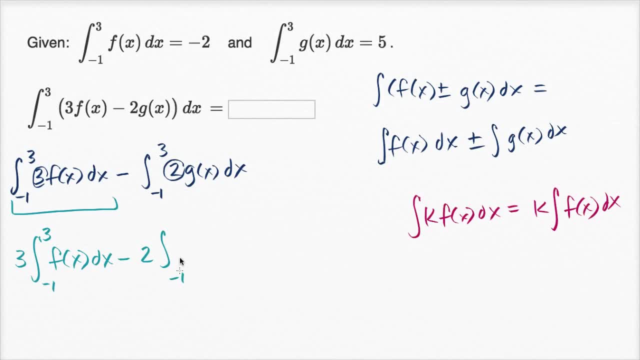 minus two times the definite integral from negative one to three of g of x. Actually, let me do the second one in a different color: Minus minus- this is gonna be in magenta- minus two times the integral from negative one to three. 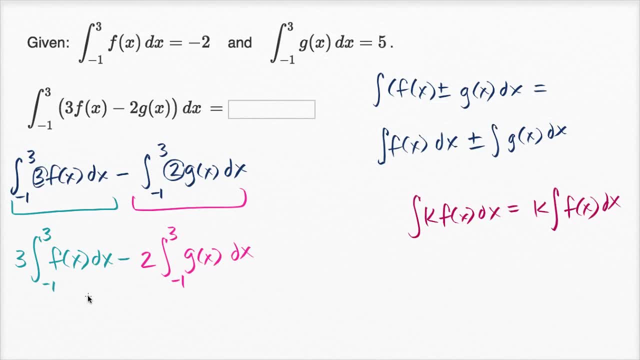 of g of x, dx. and so what is this going to be equal to? Well, they tell us. they tell us what this thing is here that I'm underlying in orange: The integral from negative one to three of f of x, dx. 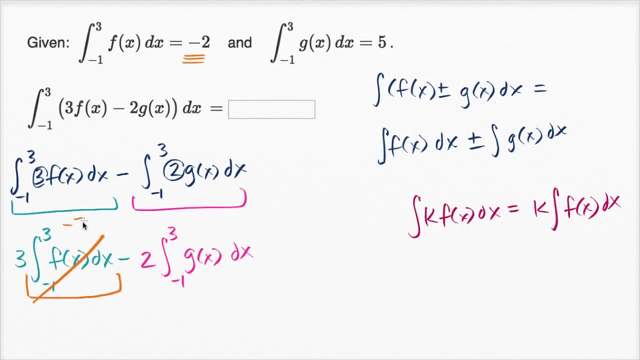 they tell us that that is equal to negative two. So that thing is negative two and likewise this thing right over here, the definite integral from negative one to three, of g, of x, dx. they give it right over here: it's equal to five. 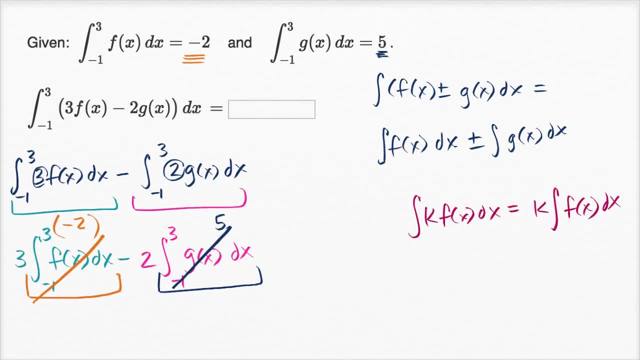 So that's equal to five. and so the whole thing is going to be three times negative two, which is equal to negative six minus two. times five minus 10,, which is equal to negative 16. And we're done.